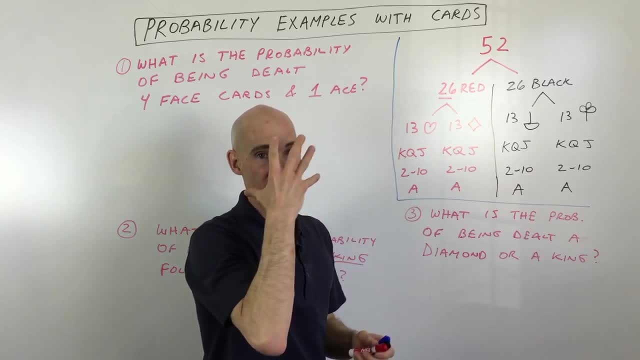 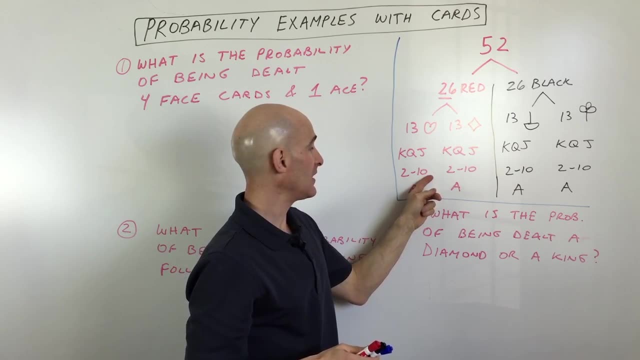 13 hearts into three face cards, so they have a face on them. They're kings, queens and jacks, okay. And then you've got the numbered cards, which are 2 through 10, okay, And then there's. 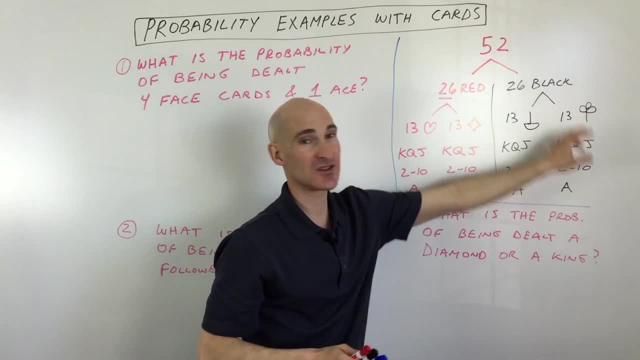 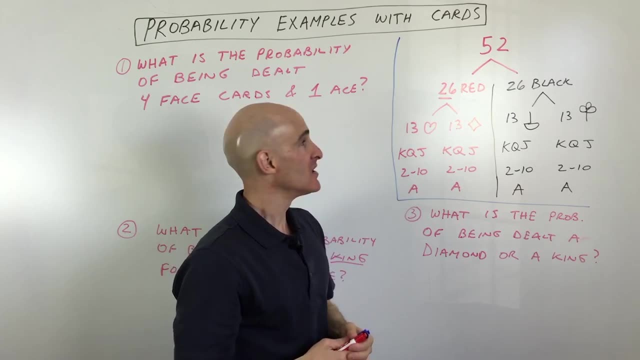 one ace. So each suit- they call these four suits, okay- of 13 cards are made up of three face cards, the numbered cards 2 through 10, and then the ace. Okay, so let's get into some examples. 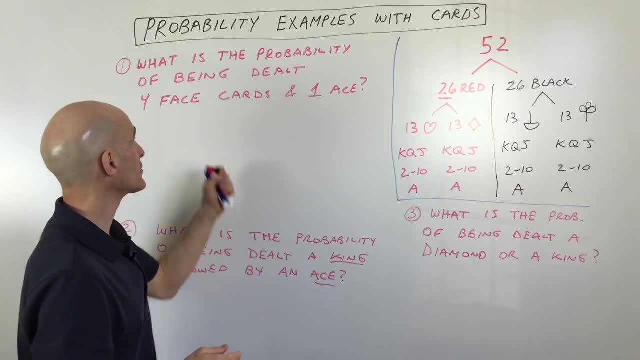 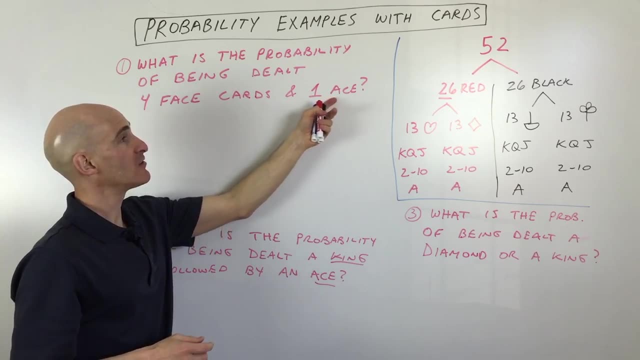 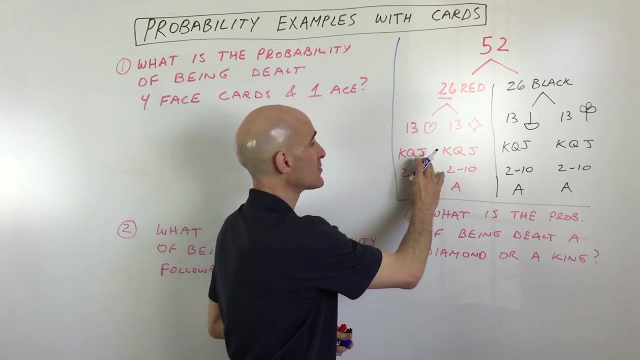 and I'll show you how to work with some probability examples here using playing cards. The first one says: what is the probability, The probability of being dealt four face cards and one ace. Okay, so that's an interesting question. So first we have to analyze how many face cards there are, and you can see there's 3,. 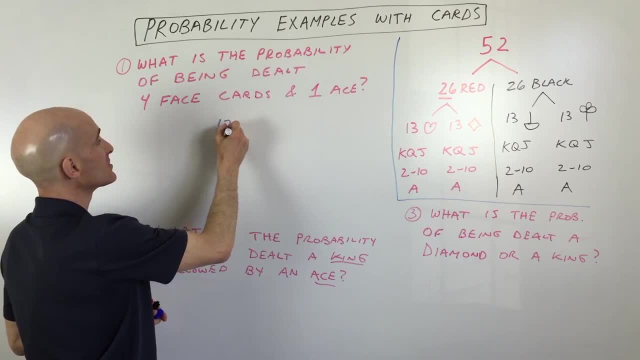 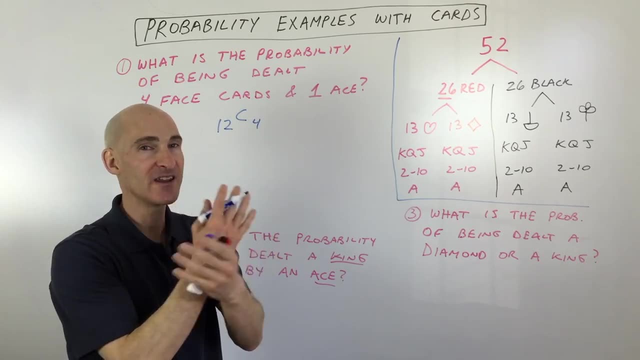 6,, 9,, 12.. So, out of 12 face cards, okay, we're choosing four. Now, the reason I'm using combinations is because when you're dealt these cards, when you hold them in your hand, it doesn't. 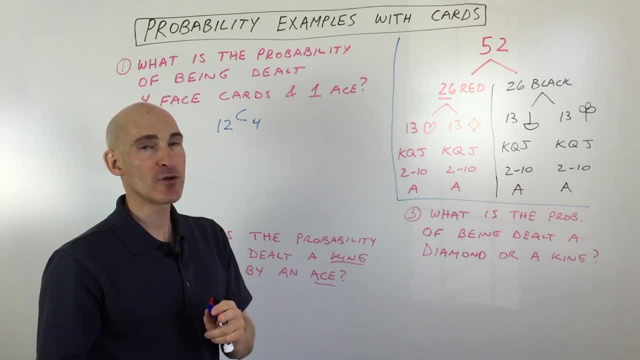 matter. you know what order they're dealt to you, So we don't want to use permutations, We want to use combinations, because the order is not important, And we're going to multiply this by all the different ways to get one ace. Now there's an. 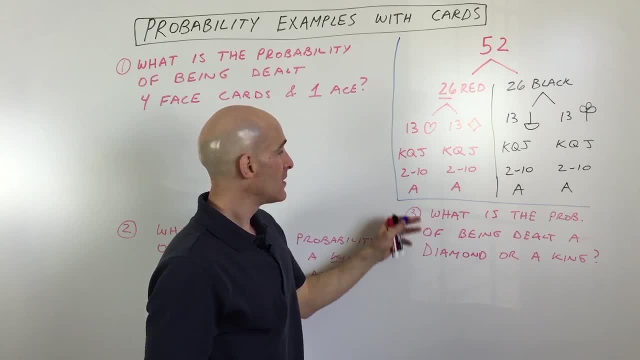 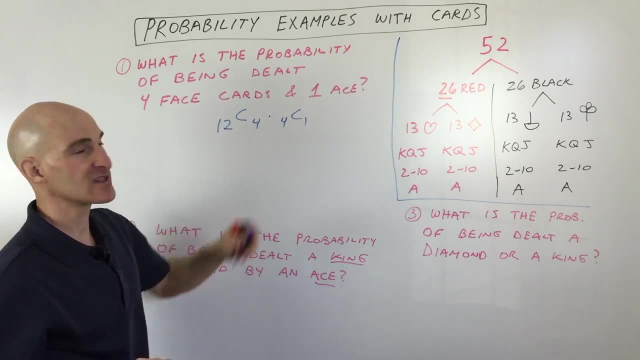 ace of hearts, diamonds, spades and clubs. So, out of the four aces, we just want to find out how many ways there are to choose one. Well, of course, there's four ways, right, But we can use it as: 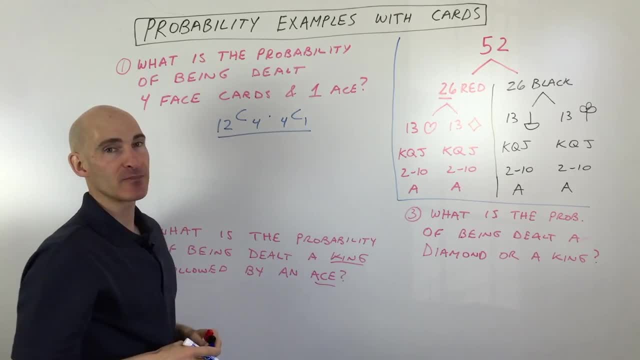 a combination, four choose one, and then we're going to divide that by the total possible five card hands. So out of 52 cards total, how many ways are there to choose five, where the order doesn't matter? So probability is the number of. 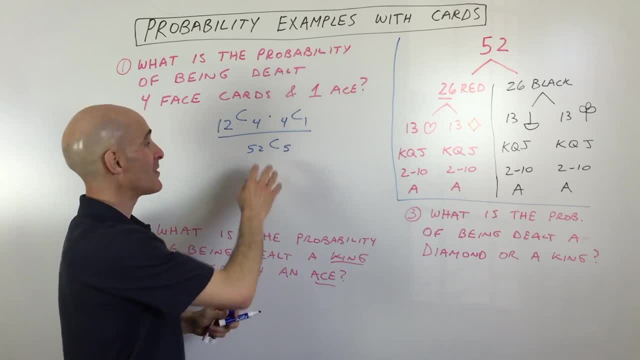 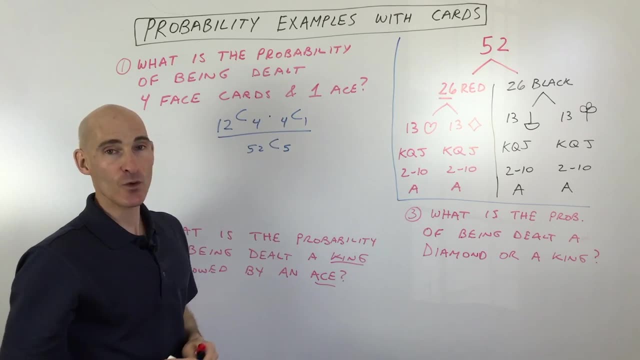 successful outcomes the number of things that you want to occur right divided by the total possible things that could occur. So if you simplify this, you know out, you're going to be able to calculate what the probability is. And just a quick note here, I'll just show you with 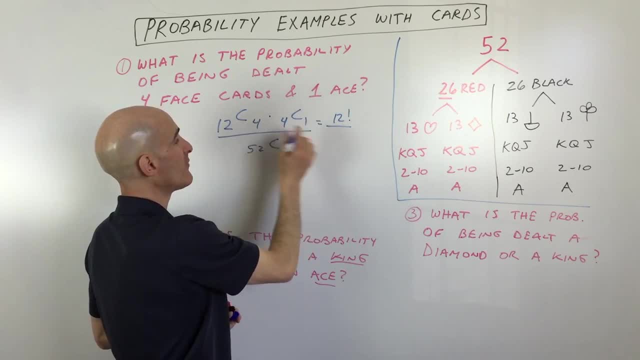 the 12. choose four. this is 12 factorial over 12 minus 4, 8 factorial 4 factorial 4. choose one is 4 factorial over 4 minus 1, 3 factorial 1 factorial, all divided by 52.. 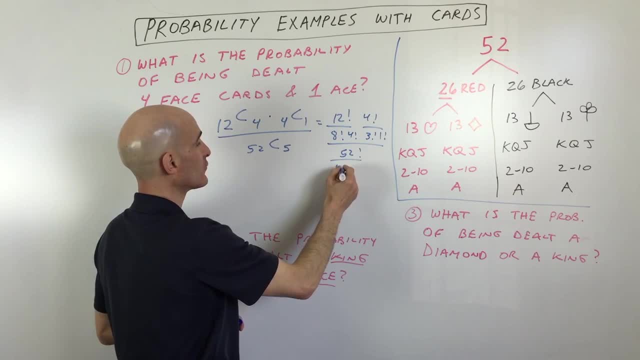 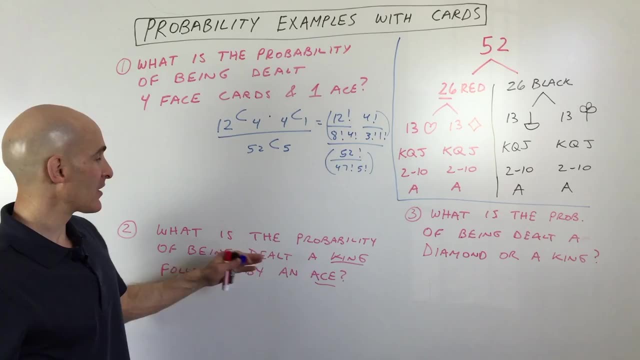 52 factorial, 52 minus 5, which is 47 factorial, 5 factorial. So if you simplify that, you're going to get the probability Okay. let's look at another example. It says what is the probability of being. 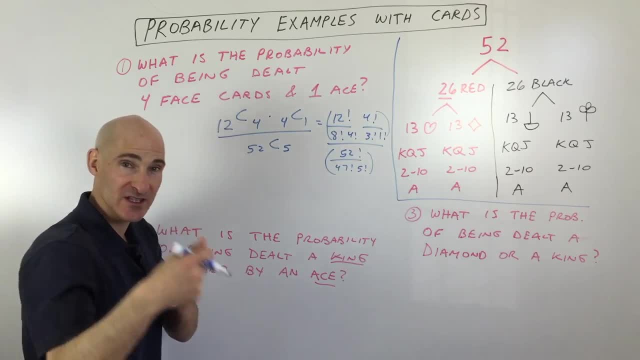 dealt a king followed by an ace, So you're basically being dealt one card and then another card. It's like reaching into a hat. What's the probability? I pick this out, set it aside, pick another card. Now, the thing to notice here is that it's not like you're shuffling that card back into. 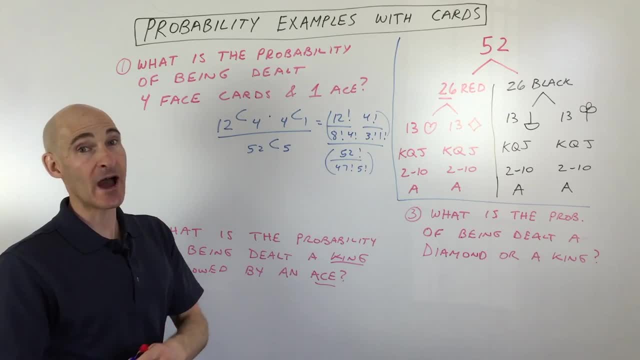 a hat. So there's this concept of with replacement or without replacement. So this is without replacement, okay, which means that these events are dependent on one another, as opposed to, when you shuffle it back in, they would be independent. The probabilities would be restored to the. 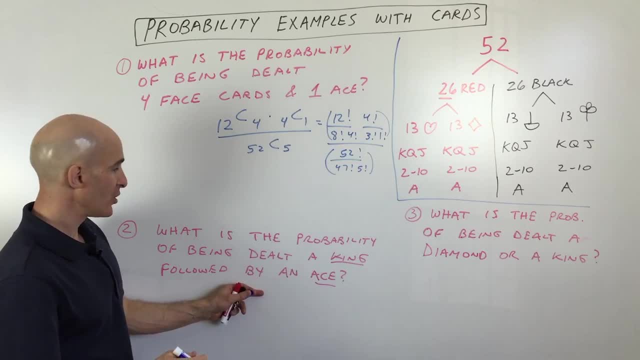 original probabilities. So what we're going to do here is we're going to look at- hmm, probably being dealt a king. Well, there's four kings, okay, and there's 52 cards total. So the probability is four chances out of 52, right? 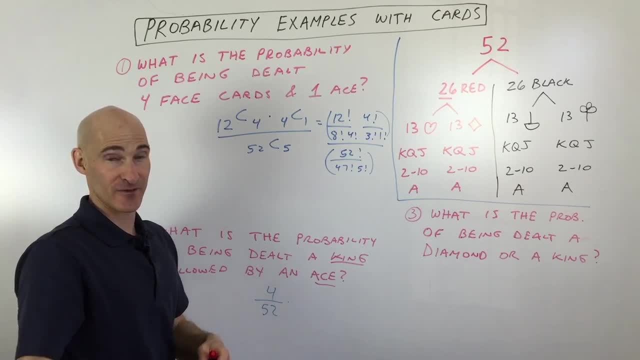 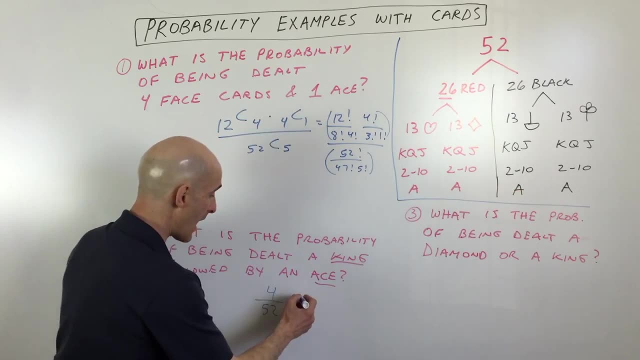 But once you're dealt that king, now what happens? There's only 51 cards left, right And we say: what's the probability of being dealt an ace? Well, you can see there's four aces out of the 51 remaining. 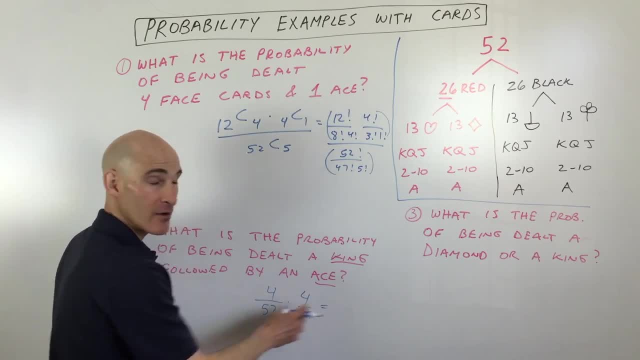 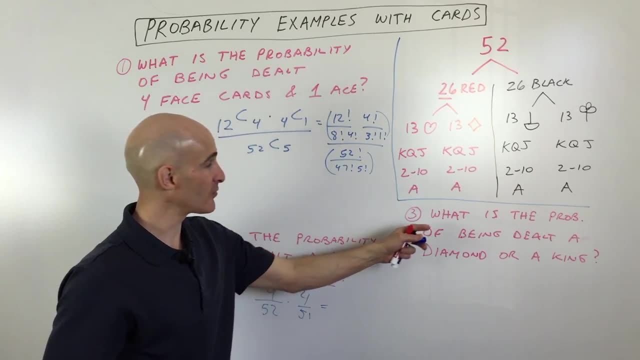 cards. So if we multiply these together we're going to get the probability. So it's 16 divided by whatever- 52 times 51 is okay. Last example, number three here: what is the probability of being dealt a diamond or a king? Now this is interesting. 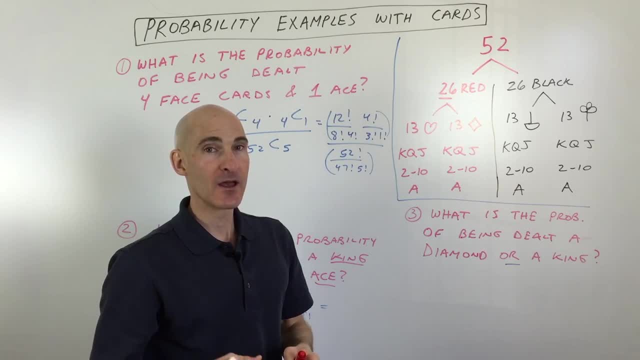 Or sometimes confuses students. in math, okay, Or in normal everyday language, means like I'm going to go to the store, I'm going to stay home, right, But in math, or means both. It means union. It means like you're combining those sets and quantities together, okay, Whereas- and you know, 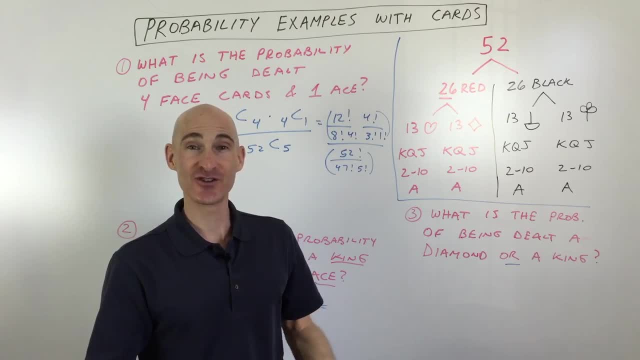 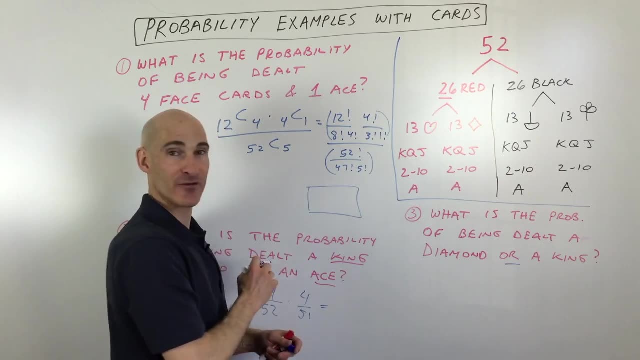 you say like I'm going to go to the store and I'm going to go to the library, It's like you're going to do both. That's everyday language In math and actually means the intersection. So if I was to draw a little Venn diagram here for you, 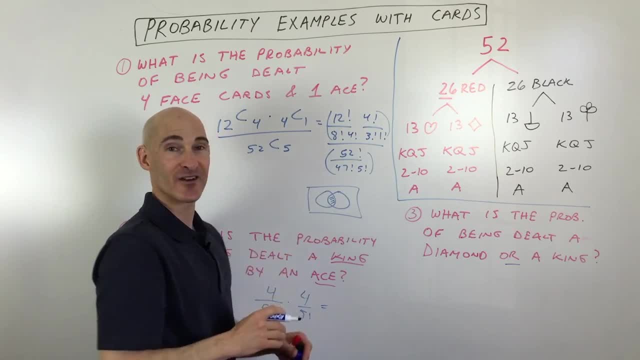 see, and means this overlapping region right there. okay, All the people that are in your math class and in your English class. okay, Like, for example, right Now, or would be like all of these people, all of these people, but you don't want to double count- the people that are in both groups. 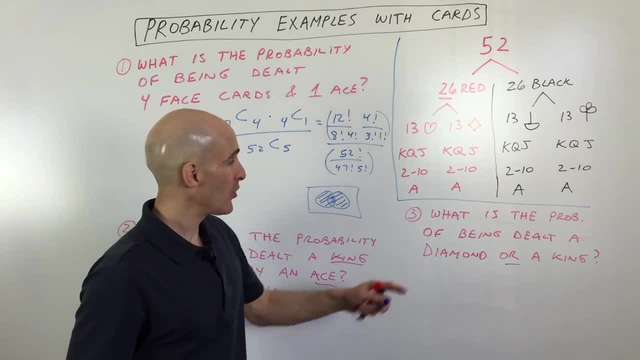 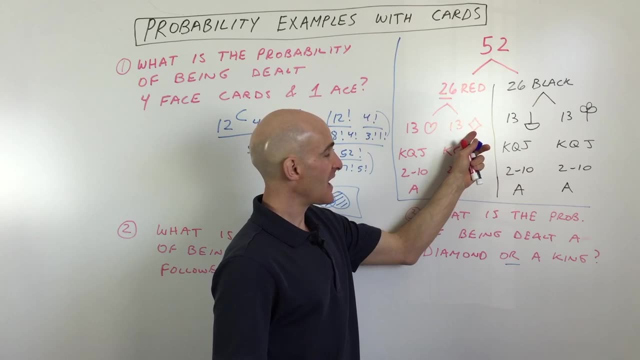 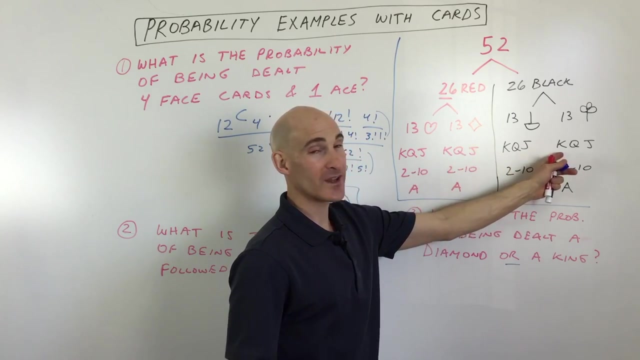 right, So you'll have to subtract off one of those double countings. Okay, so back to this problem. what is the probability of being dealt, a diamond or a king? Well, you say, hmm, 13 diamonds, right, Okay. and how many kings are there? There's four kings, but there's one. 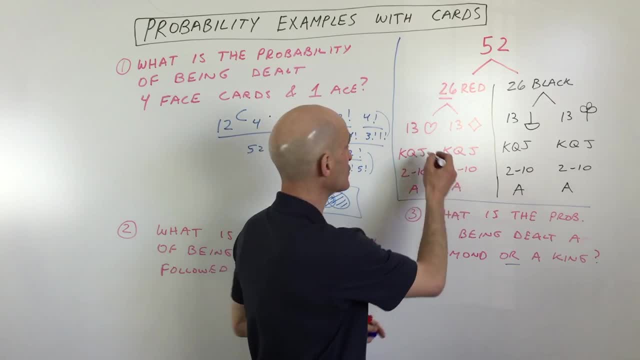 king of diamonds. Okay, so you're double counting that. So if I could just kind of circle this here to show you, like, here's the kings one, two, three, four kings, Here's the diamonds- okay, like everything that's kind of in this group, and you've got that king of diamonds that's in both. 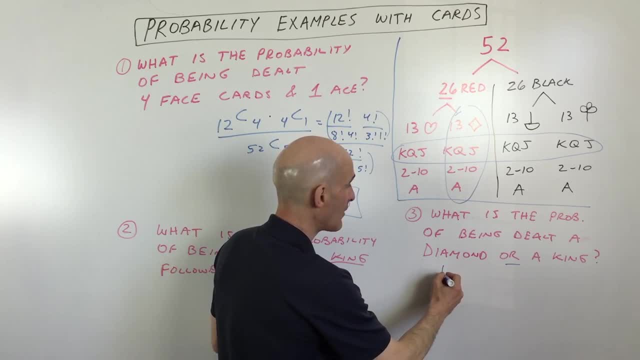 groups, So you don't want to double count it, So let's, what we're going to do is we're going to 13 out of 52, plus the probability of being dealt a king, which is four out of 52 minus the. 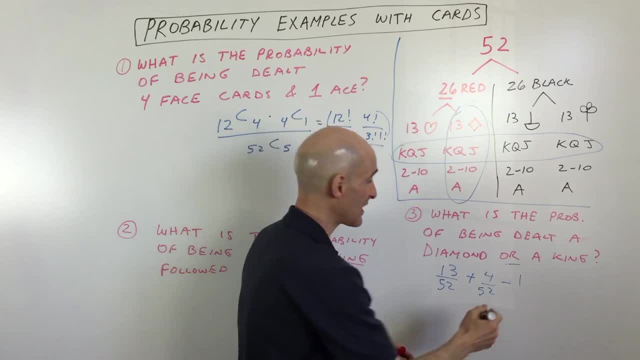 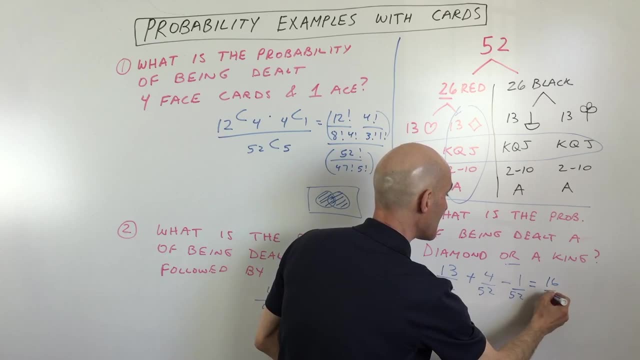 probability that you're dealt the king of diamonds. right, Because we counted that one twice, We're going to subtract the probability of being dealt the king of diamonds. So if we simplify, we get 16 out of 52, and you can reduce that further: eight out of 26, or four out of 13.. So that's.